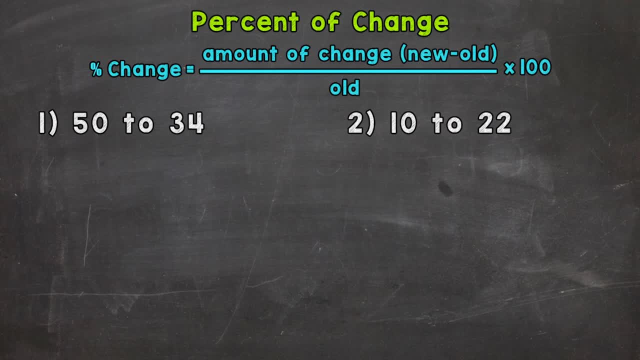 decrease there. so keep that in mind as we go through our problem. So the first thing we need to do is calculate the amount of change. So the new number minus the old number will give us that. So the new number is 34 minus the old number of 50. So 34 minus 50 gives us a negative 16.. 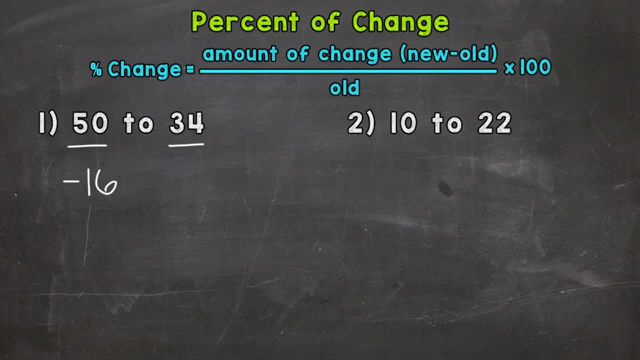 Now that negative is important because it shows us that we have a decrease. Divide that by the old or original number of 50 and then multiply by 100 to convert that to a percent. It's very important to always divide by the old or original number, because that's the number that changed. So we want 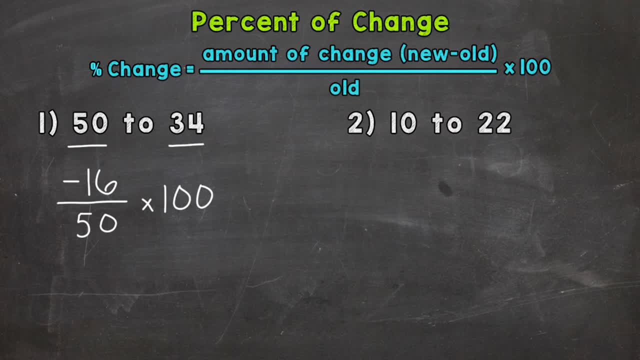 the percentage change relative to the number we started with. We're looking at the percent that we started with, All right. so negative 16 divided by 50 is going to give us a negative 32 hundredths. and then multiply that by 100 again to convert that decimal to a percent. So we can multiply. 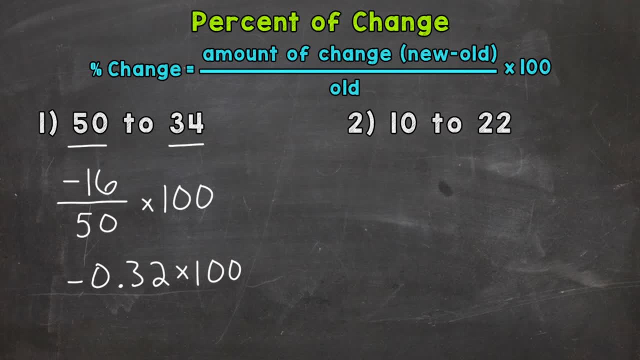 that decimal by 100 by moving the decimal twice to the right. So 1, 2, and we end up with a negative 32 percent. So we can express that answer into what we call a negative 32 percent. So we can write it in two ways, Just like what we wrote: negative 32 percent and that negative shows us. 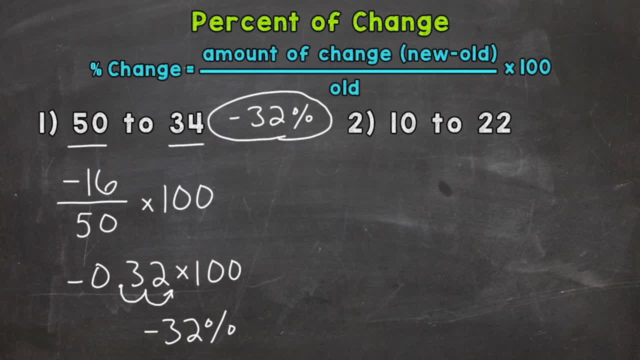 that we had a decrease. So this would be one way. Or we can write 32 percent and then the word decrease to show that we had a decrease. So 32 percent decrease or negative 32 percent. Now both of those represent that percent of change between the 50 and 34. They represent that decrease Now. 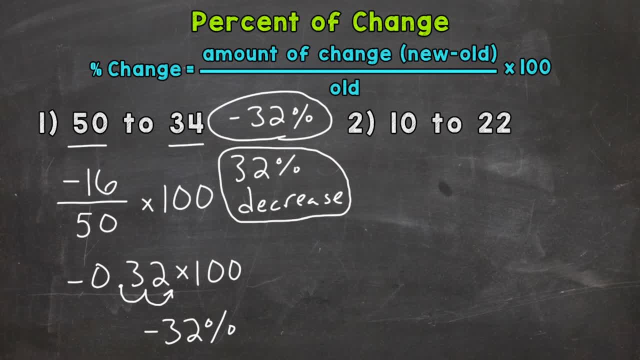 remember, whenever you see a negative, that represents a decrease. Let's move on to number 2, where we have 10 to 22.. So we can see that we have an increase there. We started with a 10 and now we have a 22.. So let's plug our numbers in and see exactly what the percent of change is. 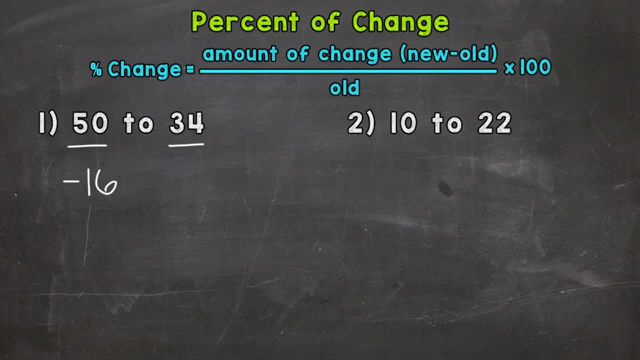 Now that negative is important because it shows us that we have a decrease. Divide that by the old or original number of 50 and then multiply by 100 to convert that to a percent. It's very important to always divide by the old or original number, because that's the number that changed. So we want 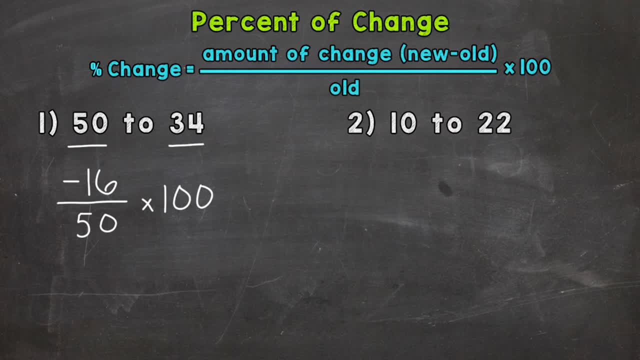 the percentage change relative to the number we started with. We're looking at the percent that we started with, All right. so negative 16 divided by 50 is going to give us a negative 32 hundredths. and then multiply that by 100 again to convert that decimal to a percent. So we can multiply. 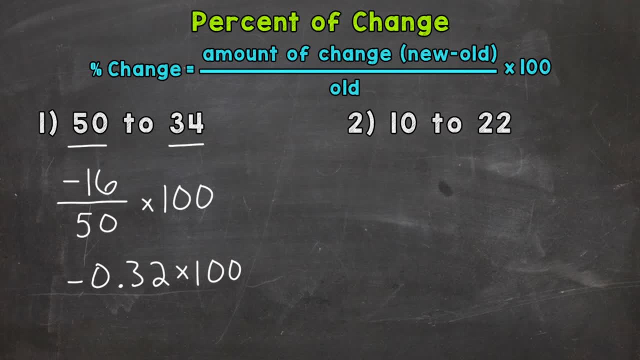 that decimal by 100 by moving the decimal twice to the right. So 1, 2, and we end up with a negative 32 percent. So we can express that answer into what we call a negative 32 percent. So we can write it in two ways, Just like what we wrote: negative 32 percent and that negative shows us. 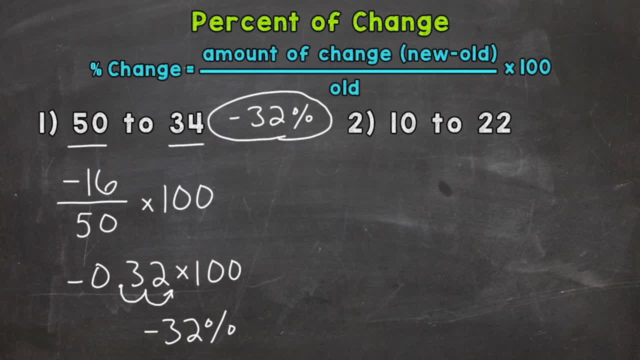 that we had a decrease. So this would be one way. Or we can write 32 percent and then the word decrease to show that we had a decrease. So 32 percent decrease or negative 32 percent. Now both of those represent that percent of change between the 50 and 34. They represent that decrease Now. 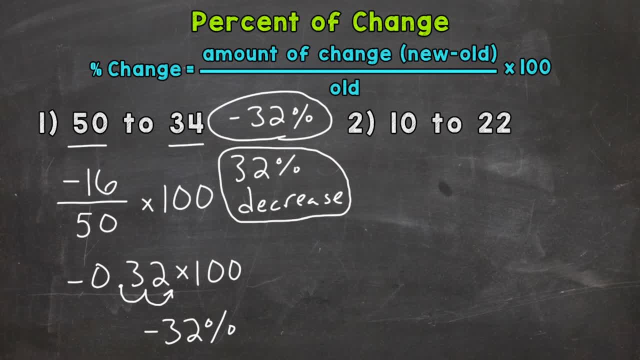 remember, whenever you see a negative, that represents a decrease. Let's move on to number 2, where we have 10 to 22.. So we can see that we have an increase there. We started with a 10 and now we have a 22.. So let's plug our numbers in and see exactly what the percent of change is. 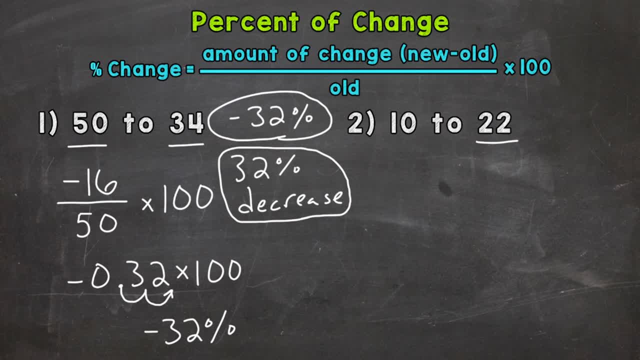 So the new number is 22.. Subtract the old to get the amount of change. So we're going to get 22 minus 10 is 12.. Divide by the old or original number of 10 and then multiply by 100 to convert that to a percent.